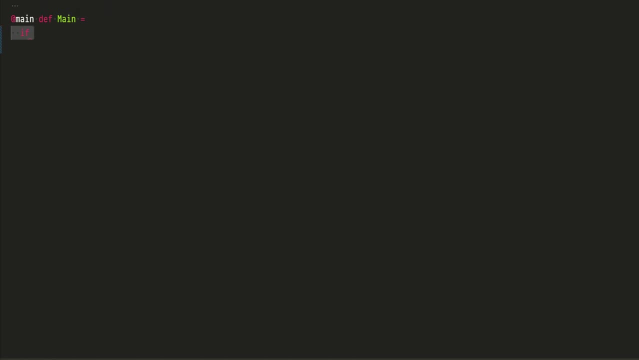 programming In Scala. we express conditions using the if statement. The if statement is followed by the condition. The condition is followed by then keyword. After the then keyword, you write what needs to happen. If that condition is true, then you can optionally write the else statement, followed by what needs. 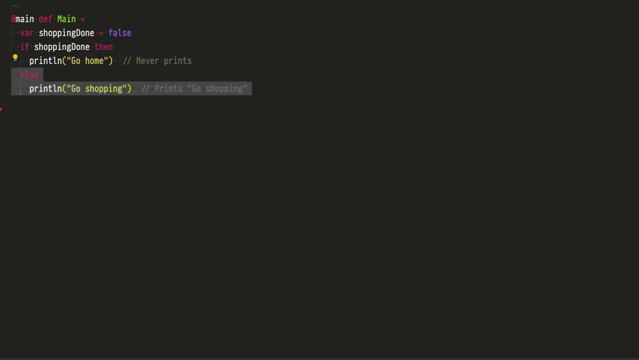 to happen. If that condition is false, the program will always follow either the then branch or the else branch. You can flip the condition for the program to follow the other branch. Multiple conditions can be unified into one condition. For example, in Scala you can express the condition. 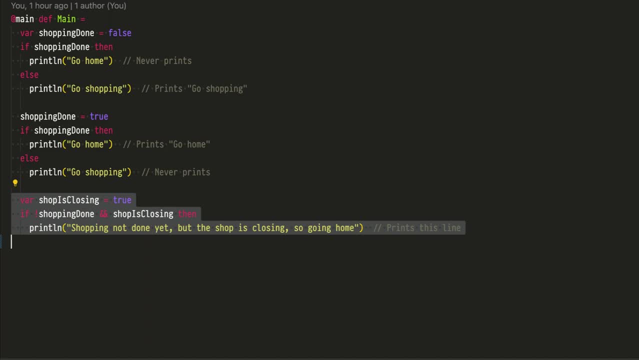 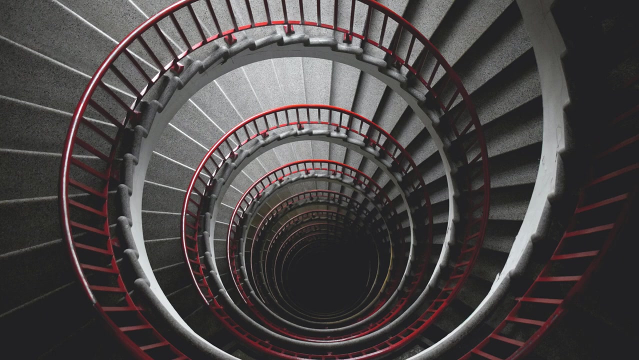 if the shopping is not yet done but the shop is closing, The exclamation statement gives you a sign before the condition negates the condition. The double ampersand operator is read as an AND operator, Another construct that is frequently encountered in programming. 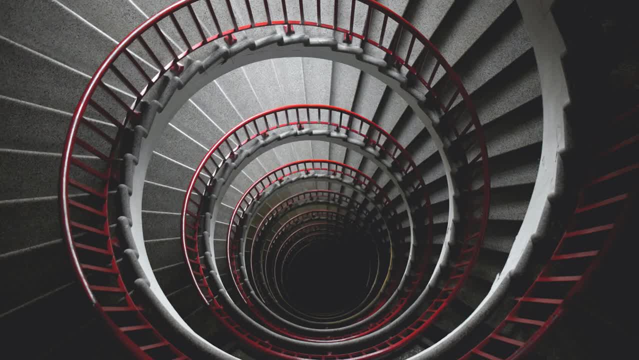 is a loop. A loop needs to be executed over and over again until a certain condition is met. In Scala, we have a while loop to do so. A while loop is started using the while keyword Joni Howele University of Michigan. AI University. 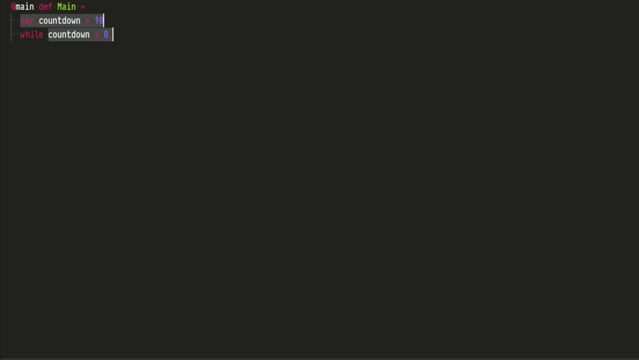 провΣtronical schwierig milenial Gu셨어요. loop is followed by a condition. As the name suggests, the code in the loop will be executed while the condition is truthful. The condition is followed by the do keyword After the do keyword. 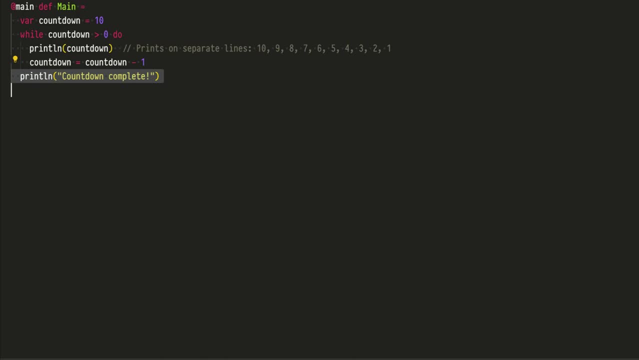 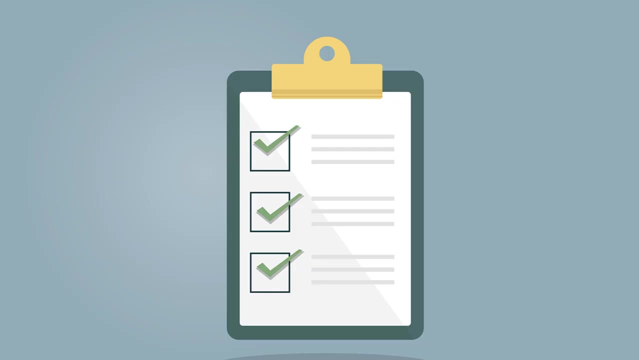 you write the code that needs to be executed in the loop. Note that only the identity code is a part of the loop. The printlnCountdownComplete statement is not a part of the loop. Another important concept is that of a list. A list is a data structure that contains multiple items of. 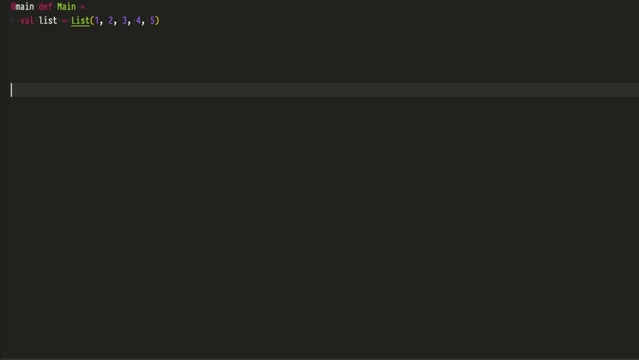 a certain type. This is a list of numbers from one to five. There are a lot of things you can do with a list. You can use foreach method defined on a list to execute code for each item of a list. For example, you can use foreach to print every item of a list You may be familiar. 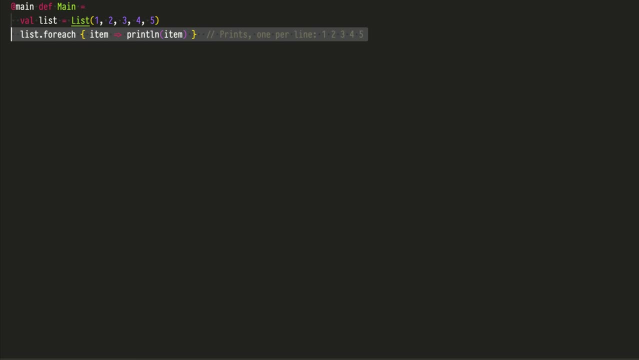 from other programming languages. with the for loop In Scala, the foreach method replaces the for loop. In Scala, the for each method replaces the for loop. In Scala, the for each method replaces the traditional for loop. Besides executing logic on every element of the list, you can transform: